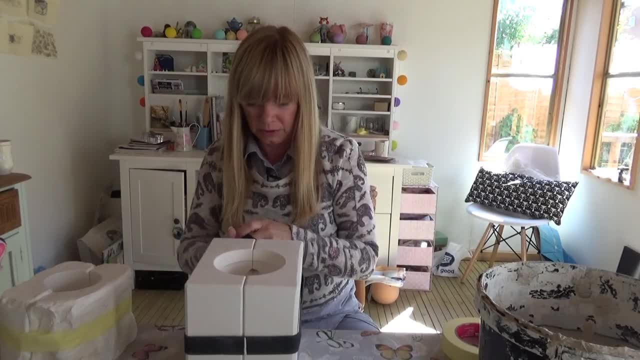 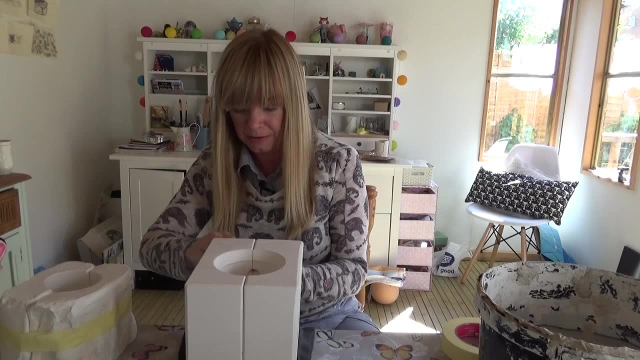 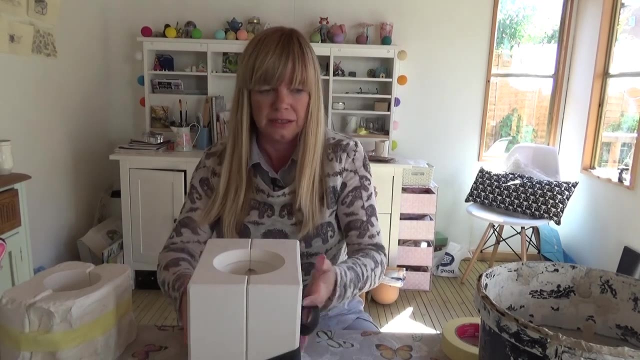 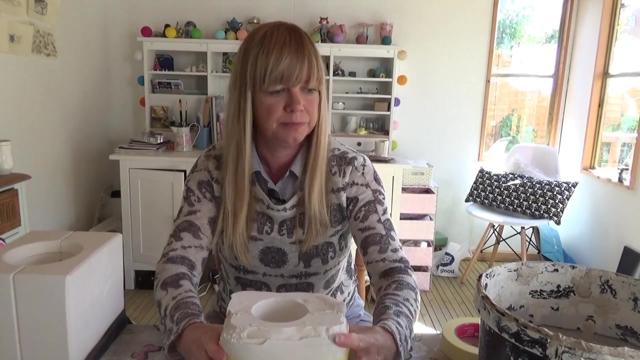 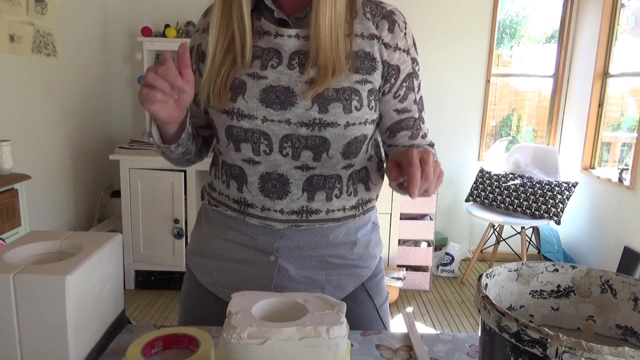 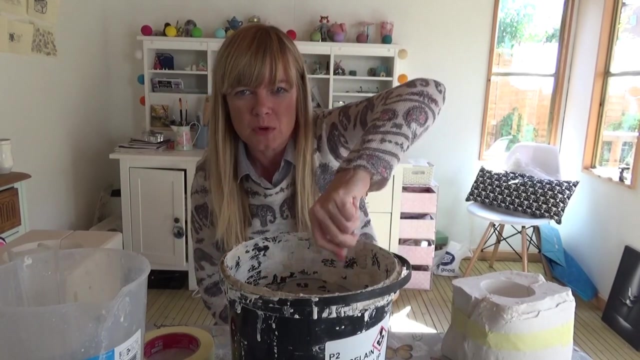 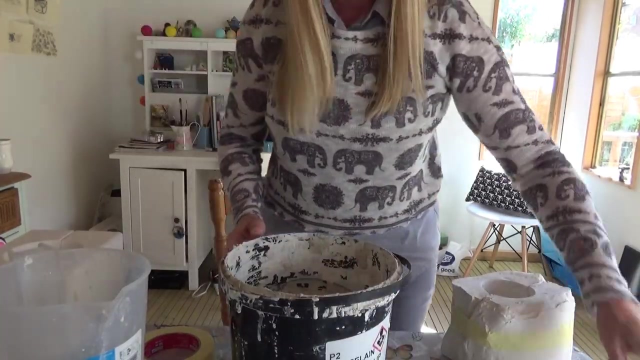 straight through and then just pull and tighten. the first one I'm going to do is this: lovely, I need to make sure that, first of all, you want to keep the porcelain. okay, you can use a picture. if you want points on the picture, you can, I think. 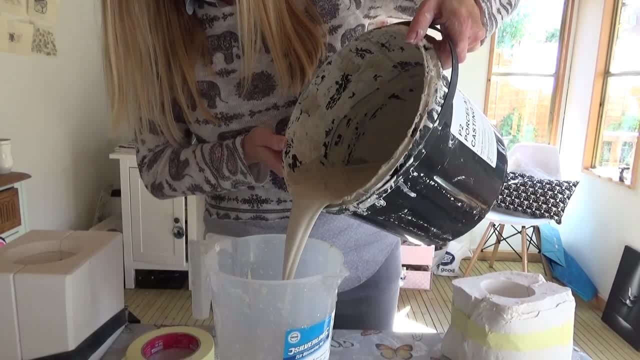 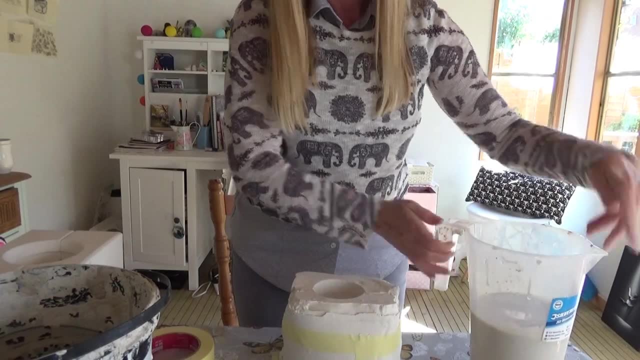 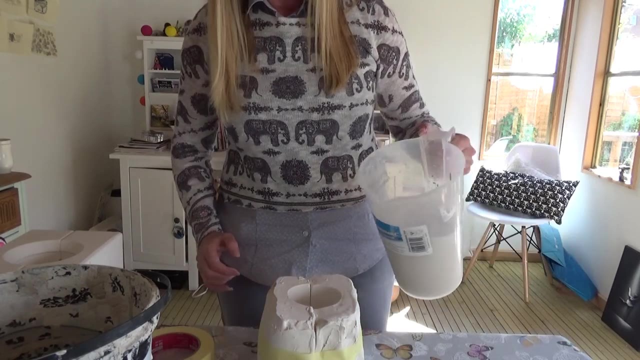 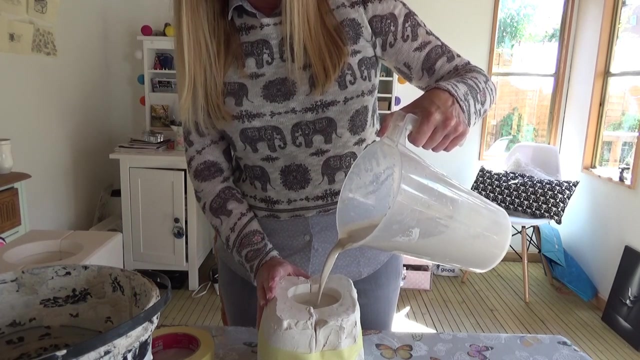 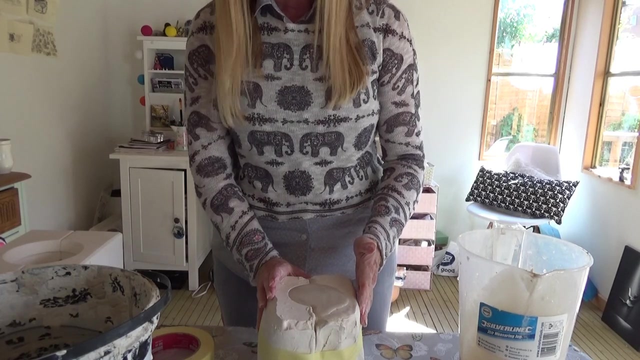 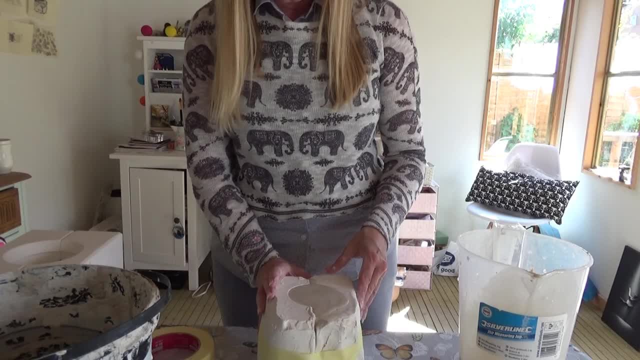 points on the picture. you can. I think now I'll leave that there for about six points on the picture, you can. I think now I'll leave that there for about six minutes and it will start to come away from the. now I'll leave that there for about six minutes and it will start to come away from the. 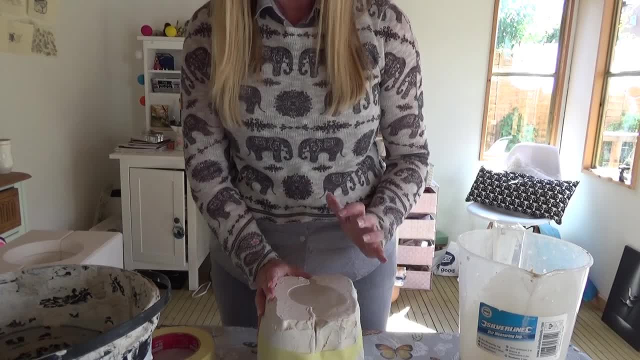 now. I'll leave that there for about six minutes and it will start to come away from the edge. or it'll start to build a wall and minutes and it will start to come away from the edge, or it'll start to build a wall and minutes and it will start to come away from the edge, or it'll start to build a wall, and that's when you'll know it's ready to tip. edge. or it'll start to build a wall, and that's when you'll know it's ready to tip edge, or it'll start to build a wall, and that's when you'll know it's ready to tip back upside down and pull the casting slip. that's when you'll know it's ready to tip back upside down and pull the casting slip. 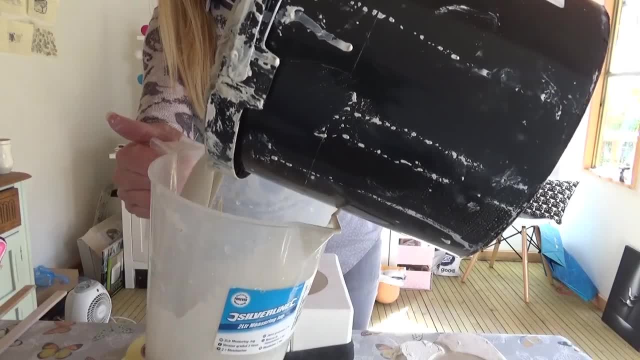 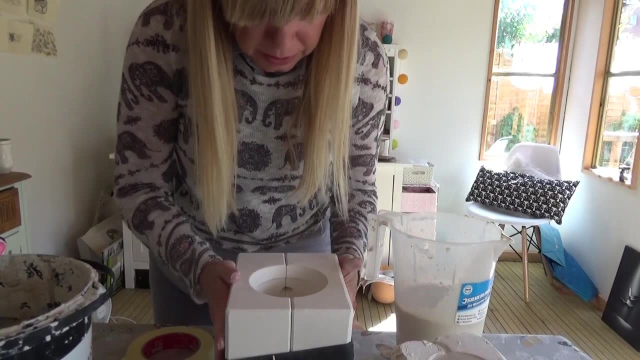 that's when you'll know it's ready to tip back upside down and pull the casting slip out should be more than enough for the look back upside down and pull the casting slip out should be more than enough for the look back upside down and pull the casting slip out should be more than enough for the look. 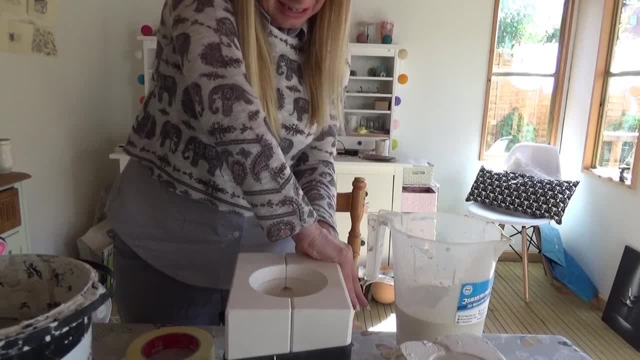 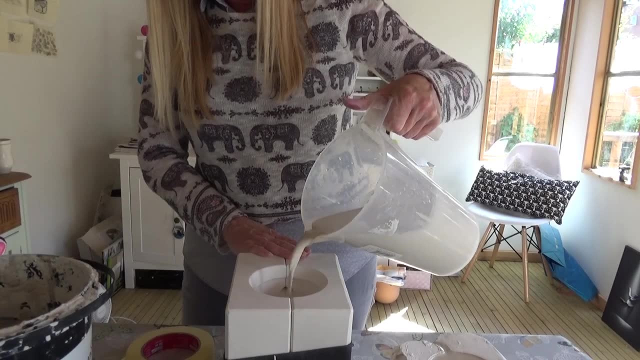 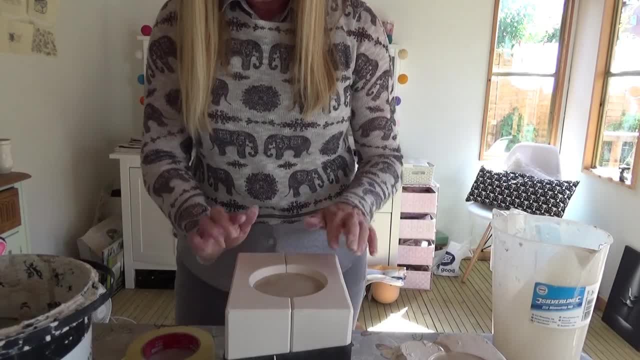 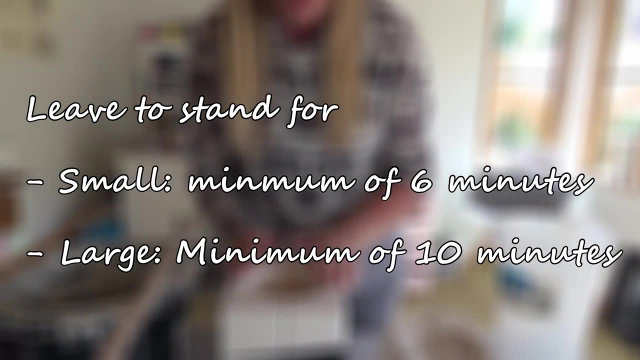 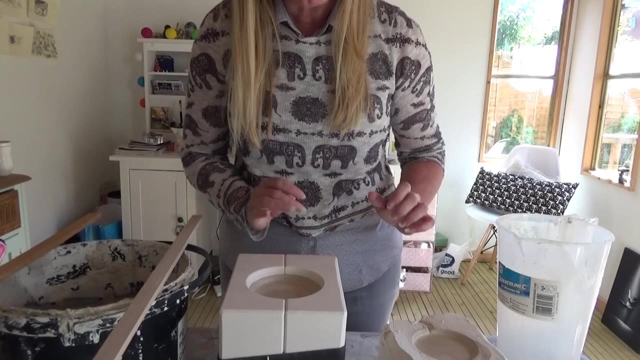 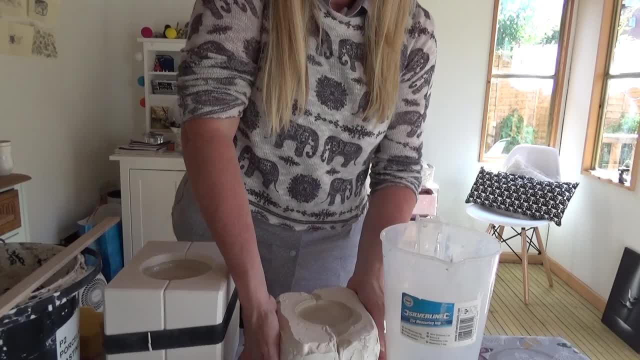 so let's pull them out. all you need is either a bouquet or a picture, either a bouquet or a picture, either a bouquet or a picture, and this fits perfectly onto the picture, and this fits perfectly onto the picture, and this fits perfectly onto the picture. so, so. 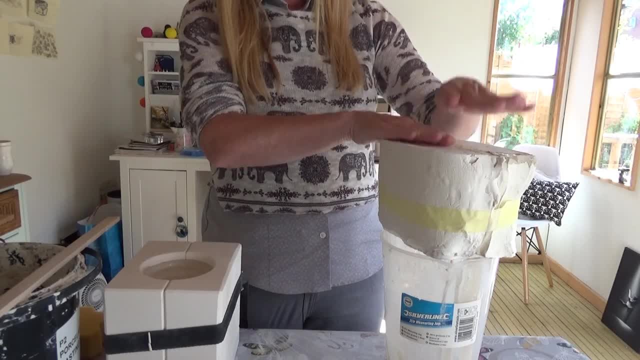 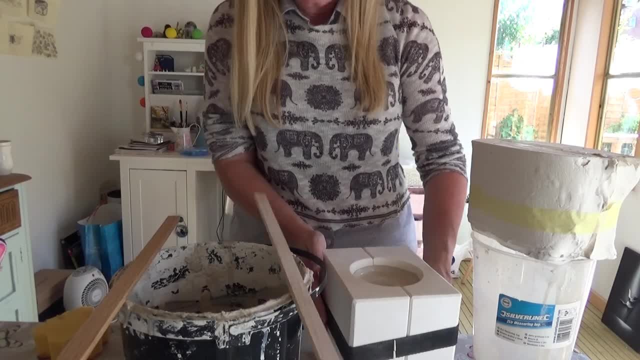 for about 30 minutes. the mug i'll leave upside down for the. the mug i'll leave upside down for the. the mug i'll leave upside down for the same amount of time. we upside down for same amount of time we upside down for same amount of time we upside down for for 30 minutes. 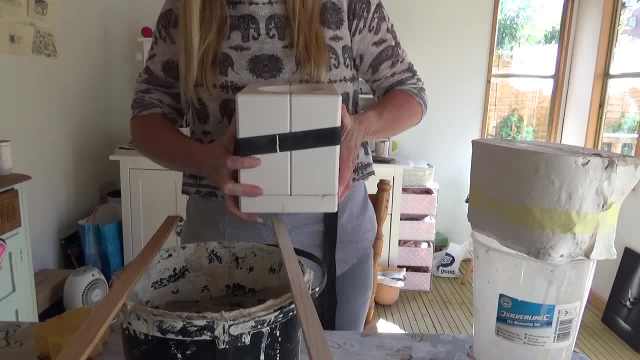 for 30 minutes, for 30 minutes. this one, this one, this one. okay, i'm gonna go. i'm gonna see if i can. okay, i'm gonna go. i'm gonna see if i can. okay, i'm gonna go. i'm gonna see if i can show you this way. 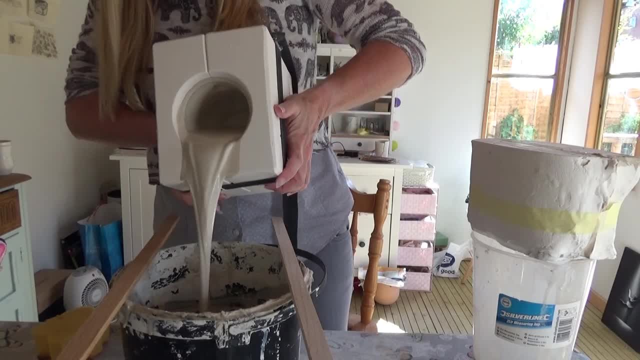 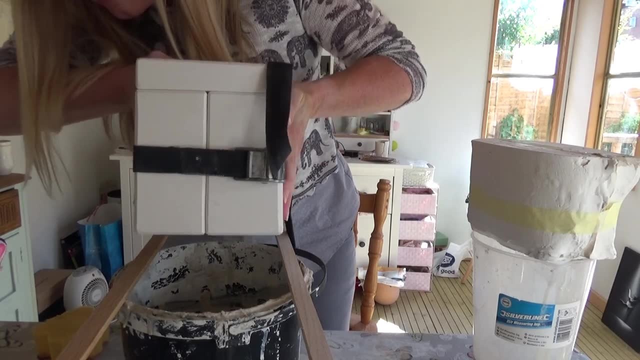 show you this way, show you this way, this one's really heavy, okay, okay, okay. let's take that upside down. and i've got, let's take that upside down. and i've got, let's take that upside down. and i've got two wooden sticks, two wooden sticks. 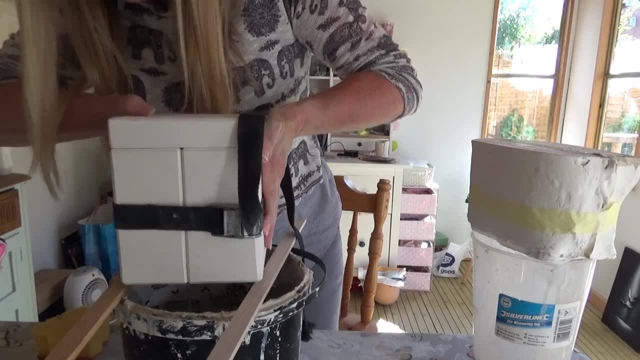 two wooden sticks. let's put this on. i just need to try and let's put this on. i just need to try and let's put this on. i just need to try and get them a bit closer. get them a bit closer, get them a bit closer. there we go, oops. 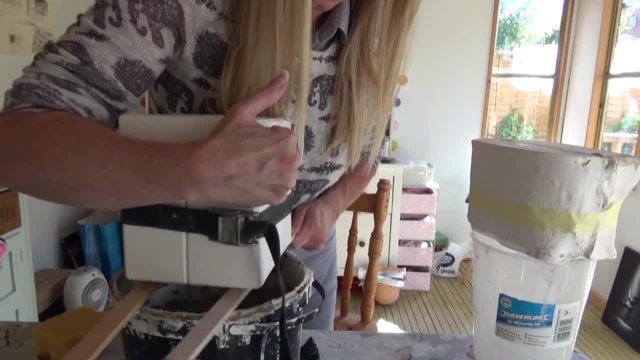 and there we go, so they'll stay upside down, and then so they'll stay upside down, and then so they'll stay upside down, and then i'll turn them, i'll turn them, i'll turn them the other way around, and then they'll be the other way around, and then they'll be. 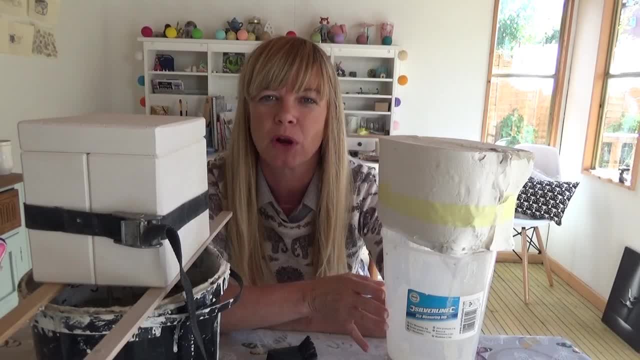 the other way around, and then they'll be left, left, left, overnight. i will do another little bit overnight. i will do another little bit overnight. i will do another little bit of a follow-on video, of a follow-on video, of a follow-on video, just to show you this. when, when, the when. 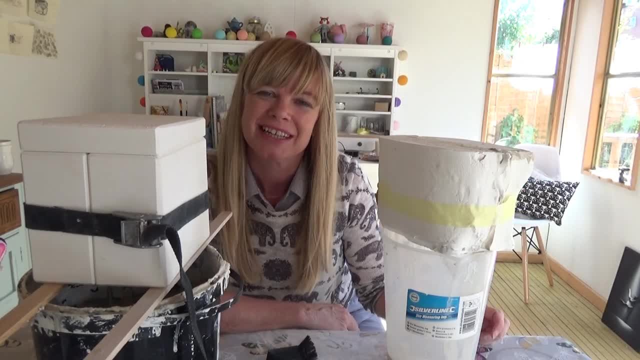 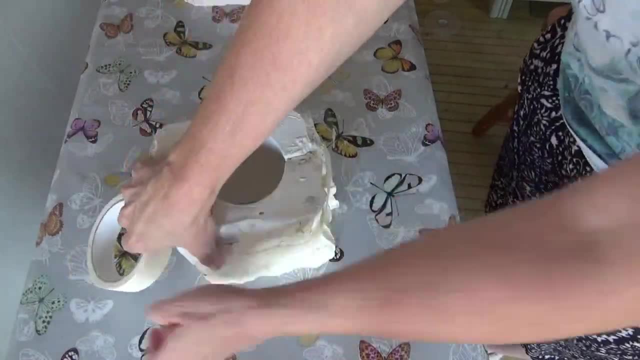 just to show you this: when, when, the when. just to show you this: when, when, the when we open the molds up, we open the molds up, we open the molds up. okay, thanks for watching and don't okay. thanks for watching and don't okay. thanks for watching and don't forget to subscribe. forget to subscribe.